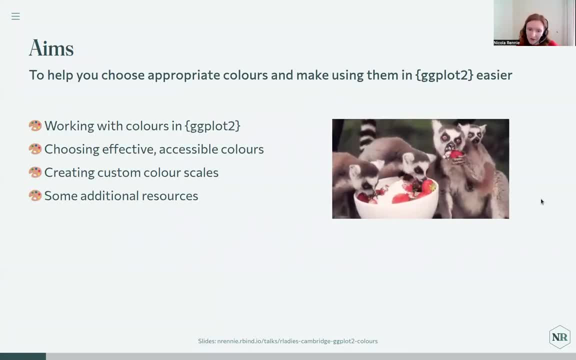 And so today I'll talk about working with colors in ggplot2, how to choose which colors to use, and then how to save yourself some time by making your own functions. I want to keep the talk sort of quite short so that we have time for discussion at the end. 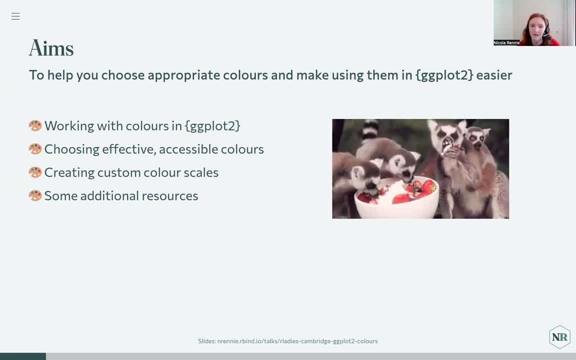 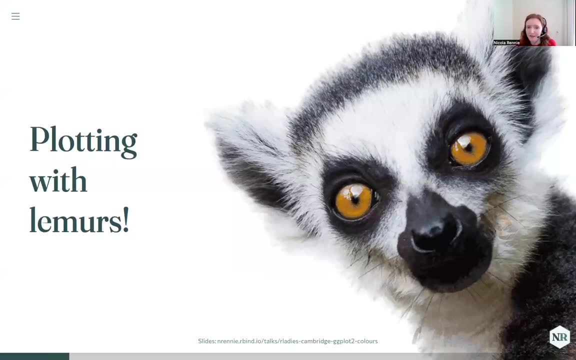 So I'll also link to some extra slides. I'll also link to some extra resources that you can sort of follow up with in your own time. So, first of all, if we're going to make some plots, we're going to need some data. I've chosen to work the examples today with some data about lemurs, and it's from one of the Tidy Tuesday data sets. 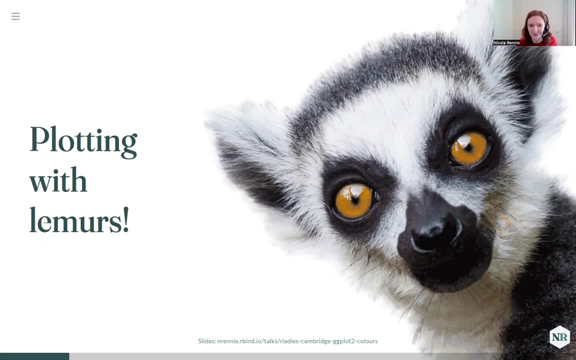 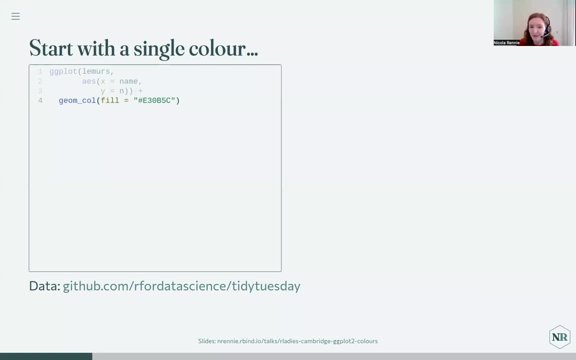 So the choice of this data set may or may not be influenced by the fact I was at the zoo yesterday. So it's a simple subset of the data I'm going to be working with. So we have just two columns: The names of some different species and n the number of lemurs in that species. 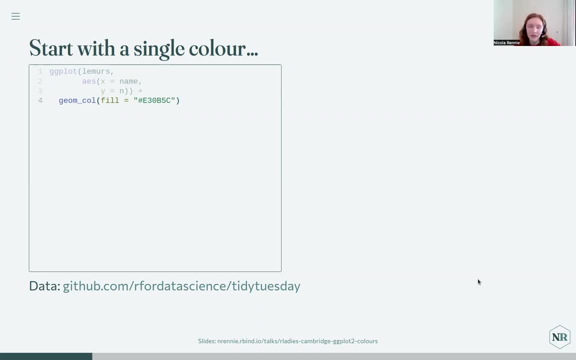 So if you're not super familiar with ggplot2, there's essentially two main ways to work with color in ggplot2.. So if we think about this example of a bar chart, here we could choose a single color for the bars, sort of independently of the data, like this, so specifying a fill color here. 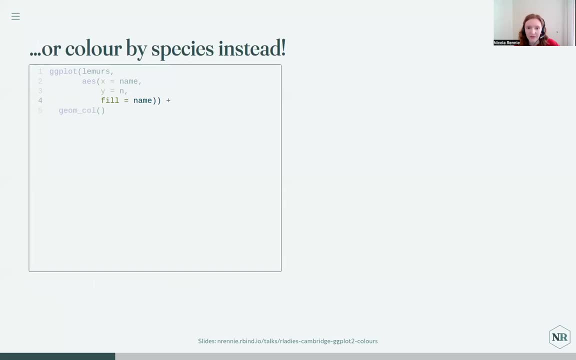 Or we could map a column in our data set to the color, so that we, in this case, get a different color for each level in that column, In this case, species of lemur, And I'm sure many of you will recognize this plot as a sort of default ggplot2 color palette. 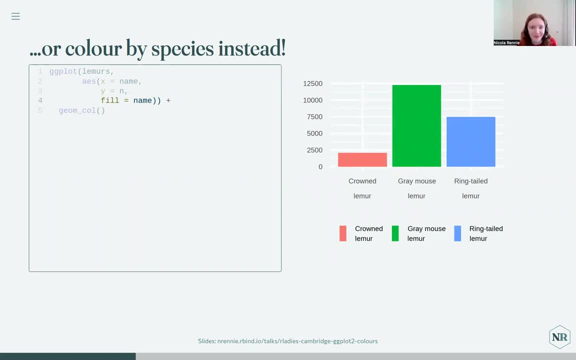 Personally, I'm not a big fan of it, And from an accessibility point of view it's not great either. It's generally not colorblind, Particularly when you start using more than three colors here. But I'll talk a little bit more about accessibility in a second. 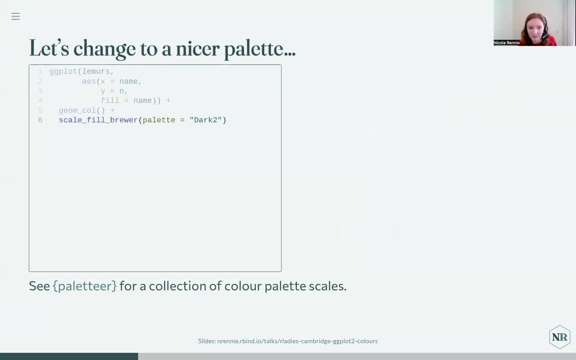 So let's change to a nicer color palette. There are some built in scale color or scale fill functions that change the colors. you see, The scale brewer functions are pretty good and there's colorblind friendly palettes in those options as well. There's also a lot of additional packages that provide even more palettes, and many of those have scale functions that you can use directly with ggplot2 or baseR if that's your thing. 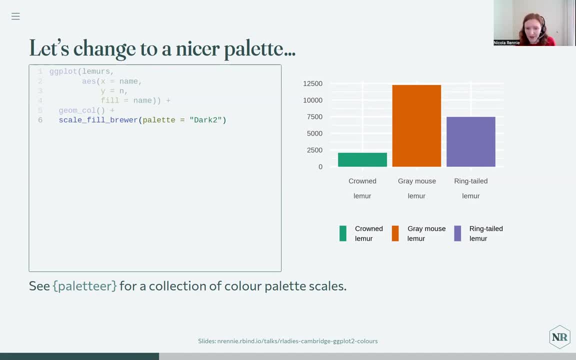 I want to point out the paletteer package here. So this is an R package that essentially collates all the other R packages that have color palettes and sort of scale functions and sticks them in one package. So it's really useful if you just want to browse through all of the potential options. 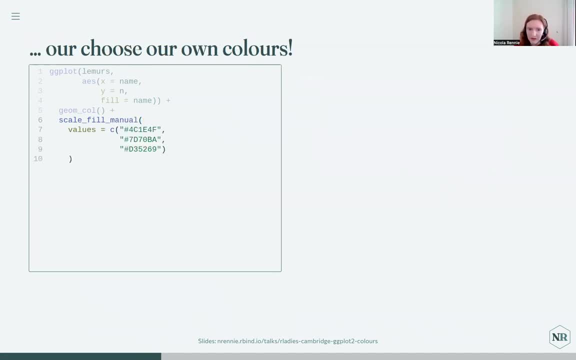 But quite often if you're working for a company who have their own color screens, or maybe you're writing your thesis and you want to make all of your plots sort of match a university logo or something, you probably won't find the exact colors you're looking for in an existing palette package that someone else has made. 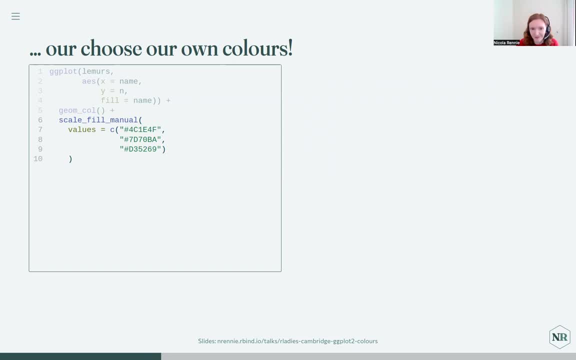 And what you can do is add your own colors with the scale, manual functions and you just pass in the text and you're done with how to do the pullout And that's pretty much it. That's pretty much it. Thanks for watching. 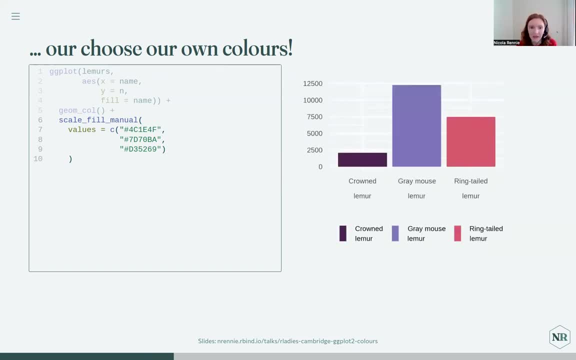 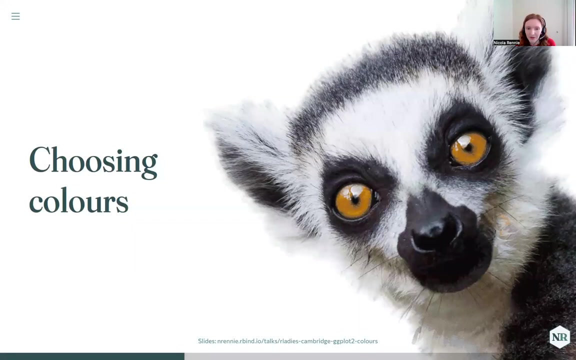 And I'll see you next time in a vector of colors that you want to use, either as hex codes, as I've done here, or as RGB values or named colors. So we know how to add colors with ggplot2, but how do we know which colors we want to? 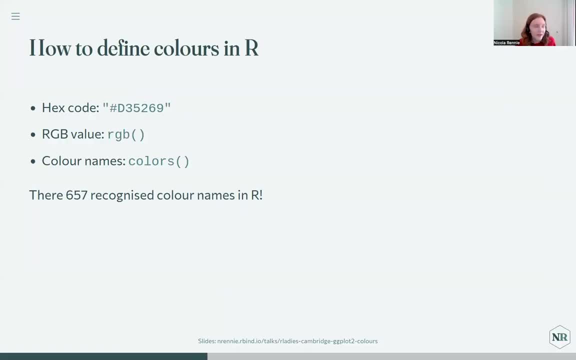 use. Well, if you think about named colors alone, there's 657 named colors in R, and then you can take into account the sort of thousands of hex codes as well. It's a lot of choice and a lot of possible combinations of colors. 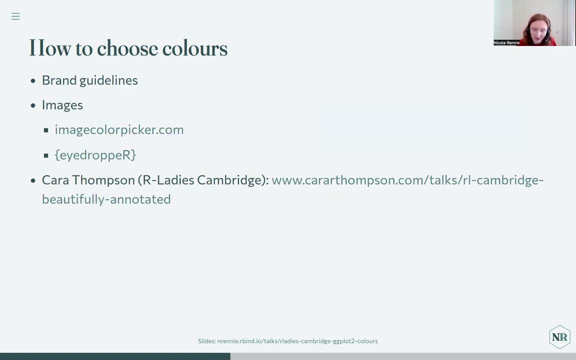 So how do we choose them? Well, if you're really really lucky, you have a marketing department in your company who has written down all of the hex codes for all of the colors you should use and in the order You should use them. 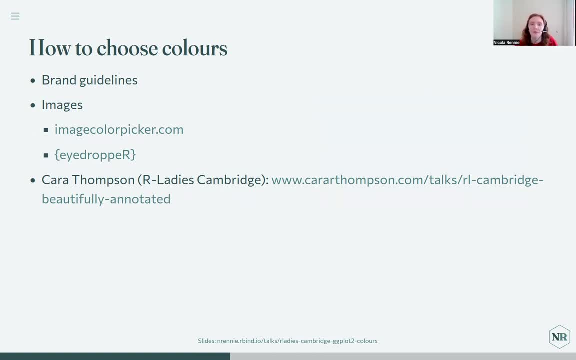 If you're not so lucky. another option is to choose colors thematically. So if you're making a plot about, say, fruit, you might want to use sort of a picture of fruit basket and pick some colors out of that. And there are some color picker tools for sort of choosing hex codes from images. 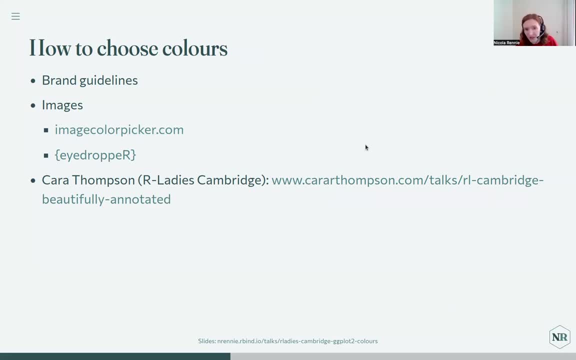 There's online tools like the image color, And there's also an R package that lets you do that directly from within R studio with the eyedropper package, which is very useful. I won't go into too much detail here. Cara did a talk last month which was really useful and sort of covered choosing colors. 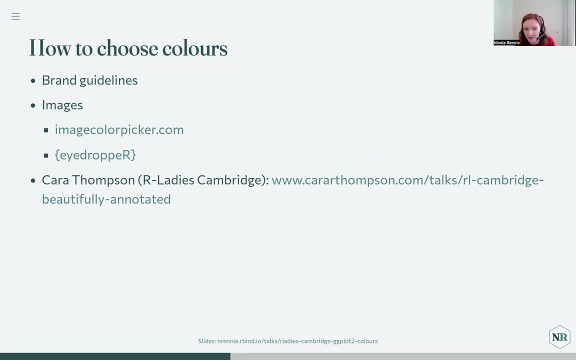 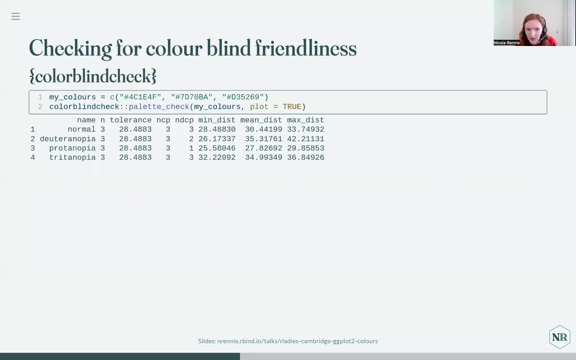 based on your data set and what your data is trying to show. So have a little look at her slides for a little bit more on thematically choosing colors. What I do want to talk about is Okay, So the first one is accessibility. 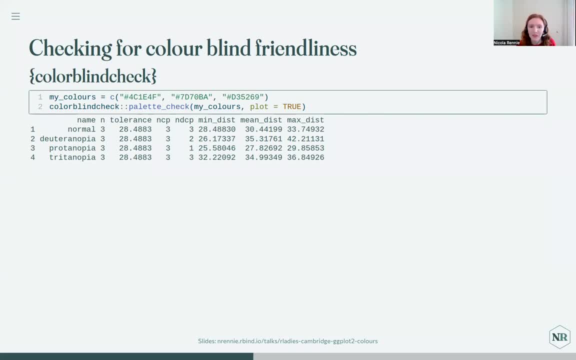 So once you've selected some possible colors, it's really important that you check if they're colorblind friendly, And there's a couple of R packages you can use to help with that. One of them is this colorblind check package, So you can pass in your vector of colors and you get this little report about your colors. 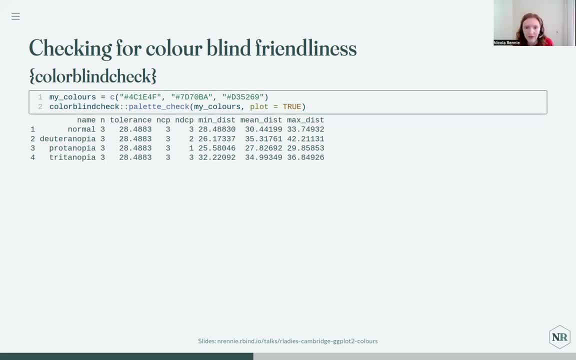 or different types of colorblindness. So here's a column I usually look at. first is this NDCP column. So that's the number of Distinct color pairs And you can compare that to the value you see if you have full color vision. 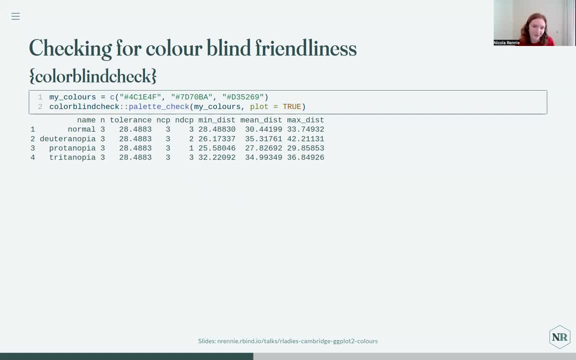 It's obviously not a sort of perfect test. It's not going to be a sort of strict this palette passes or this palette fails. You still have to sort of look at how distinct the colors are from each other, And it's usually easier to do that visually. 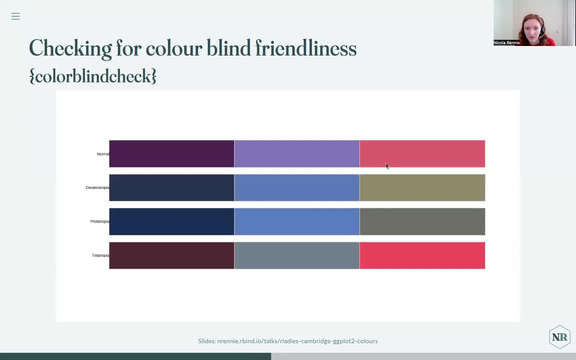 So if you also set plot equals to true, you see what the colors look like with different types of colorblindness, Which is quite useful. Now, if you want to visualize what a palette looks like with different types of colorblindness, I would also recommend looking at the colorblind R package, which transforms how the colors 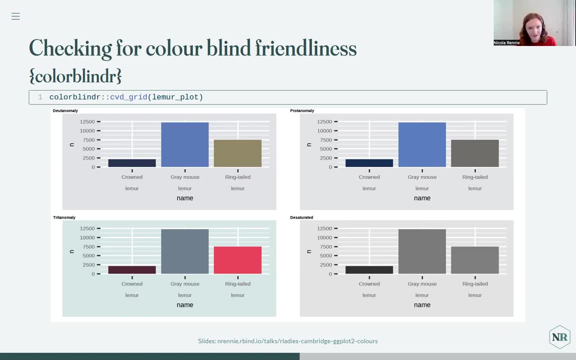 look in your plot, And the nice thing about this- rather than just sort of plotting the palette itself- is it also allows you to see what the contrast is like with the background color. So that's especially important if you're not using a sort of standard white. 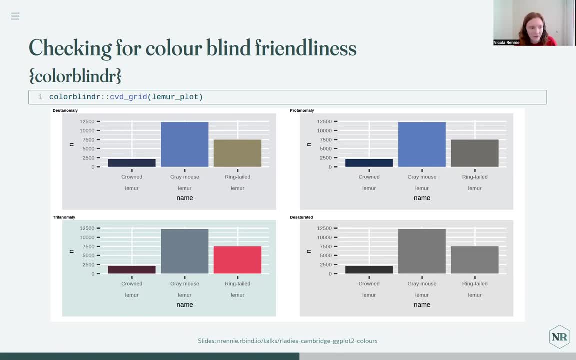 It also lets you see what the colors look like in monochrome, And this is something I wish I'd known about earlier. So here the three colors look okay-ish in terms of colorblindness. In monochrome, the last two colors are pretty much indistinguishable. 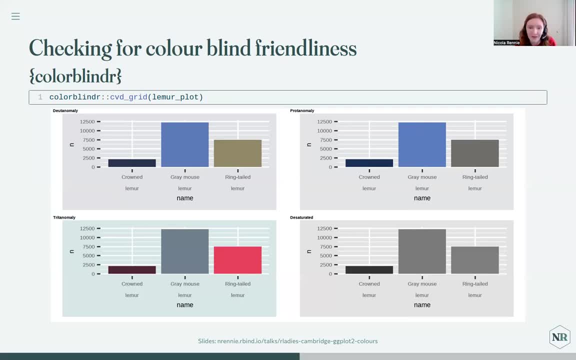 And this can be a problem for journal publications. So reviewers or journals themselves Sometimes print articles They're reviewing or publishing in black and white. So it's sort of an additional thing to check And it's something that was sort of pointed out to me in some of my plots that even though 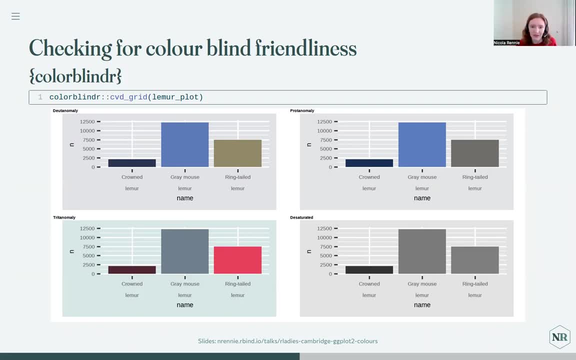 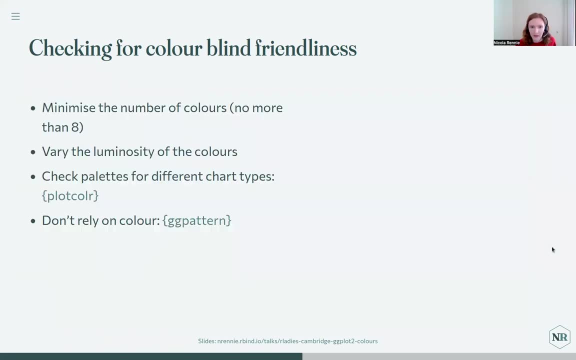 I'd picked colorblind friendly colors. they didn't work when you printed them in black and white. So, alongside these packages, there are some sort of general guidelines that are useful for helping to make colors accessible. So, generally speaking, there are some general guidelines that are useful for helping to. 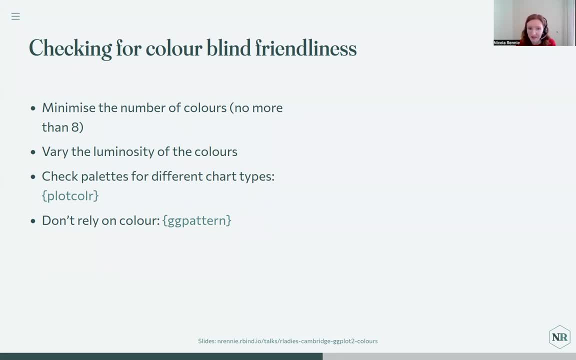 make colors accessible. Generally, you want to minimize the number of colors you're using. It's much easier to find three distinct colors than 12 distinct colors. You should also think about varying the luminosity of the colors you picked, So the brightness of the colors. 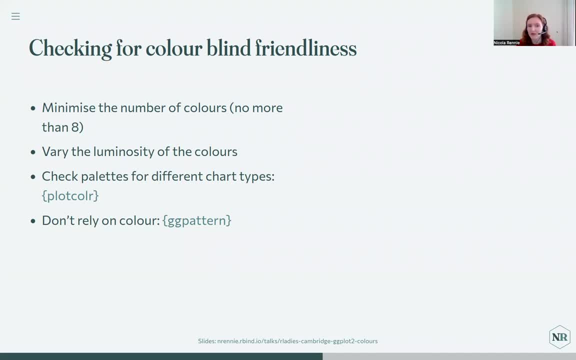 And this is one of the problems with the default ggplot2 colors. They're all equally bright, And this is also the thing that can make printing them in black and white more difficult as well. So if you're, as well as varying them in sort of hue in color, if the colors also vary in 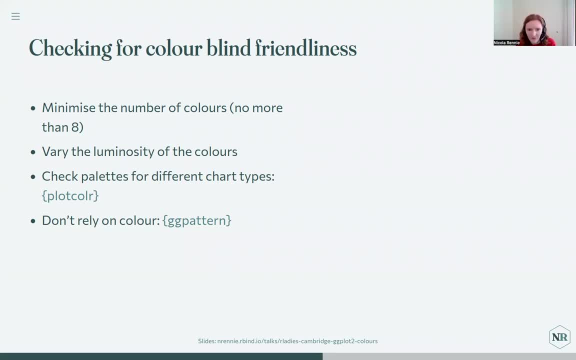 brightness. it just makes them easier to tell apart. And of course, all of this applies to not just sort of plot elements like bars or points, but also things like checking the contrast of the text against the backgrounds, And there's a few different sort of online tools you can use to check if sort of text. 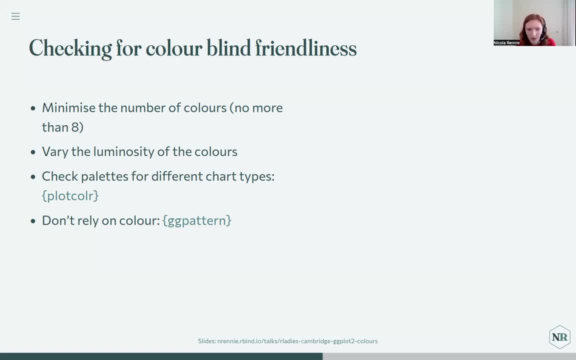 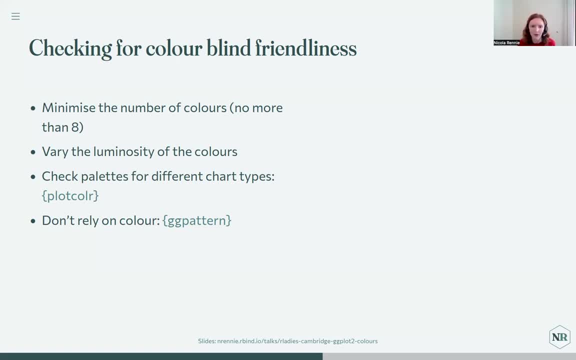 And you can also check what your colors look like on different chart types. So this plot color package lets you see what different colors look like in, say, a line chart versus a scatter plot versus a bar chart, And you might find that some particular choices of colors look okay in a map. 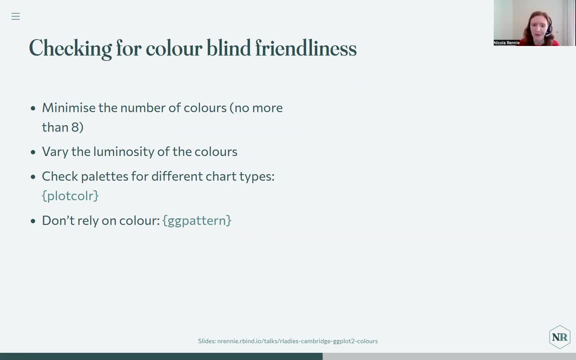 But if they're in lines and the lines are thinner, it's harder to tell them apart. And actually, despite the fact that this entire talk is about colors, the most helpful thing thing I think I could say is: don't rely on color alone. Human beings in general. 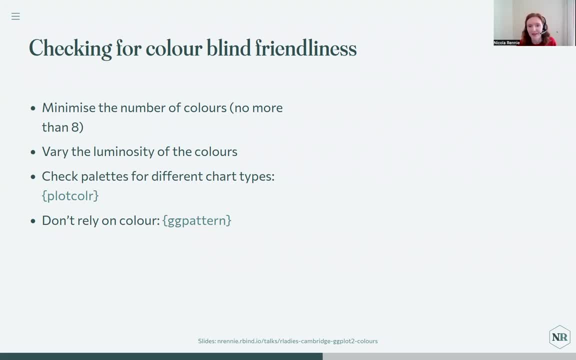 aren't always that great at interpreting colors, and then when you add in the accessibility issues, it's important to not just use color. So if you're making a scatterplot, the point should also have different shapes if they have different colors. and if it's something like a bar chart, there's a ggpattern package. 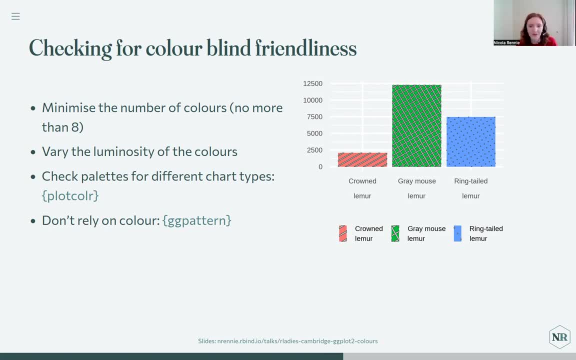 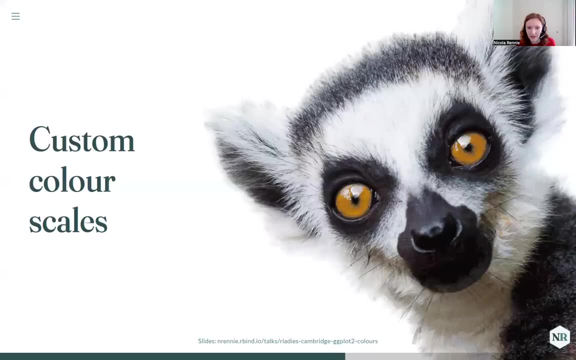 which can add patterns of dots or stripes or something to the bar charts as well as the colors themselves. So let's assume that we've picked some colors, we've checked they're accessible and we're ready to use them. We could pass our vector of colors straight into those scale manual functions I mentioned. 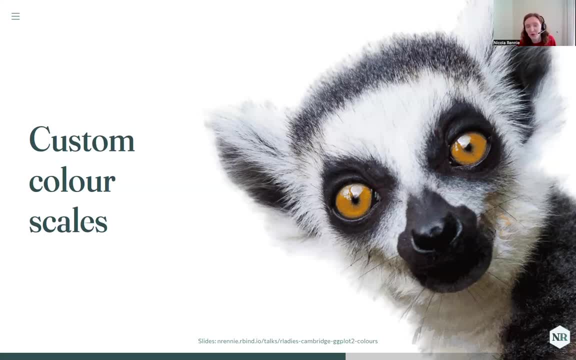 but that means that if we're making multiple plots, for example for a presentation report or something, and you want all of your plots to be styled consistently, then you've got to copy and paste that scale manual code into all of your plots. and similarly, if anyone else wants to use it, if you work in a team, in a company, you want other. 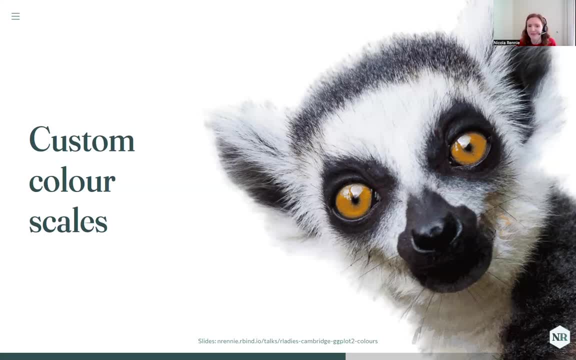 people's plots to be styled consistently as well. so again, you have to email that code back and forth and then copy and paste it, and in R we don't really like copying and pasting right, so instead we can make our own scale functions. So the first thing I'm going to do is store my colors and 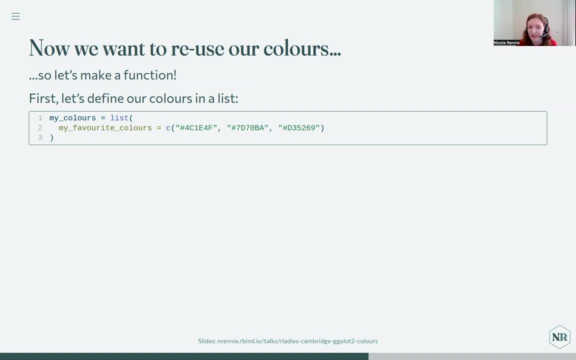 then I'm going to put them in a list. This makes it easier if I want to have multiple palettes, so I might have a sort of sequential palette and then I have a discrete palette here, for example. so here I've just gone for one and I've 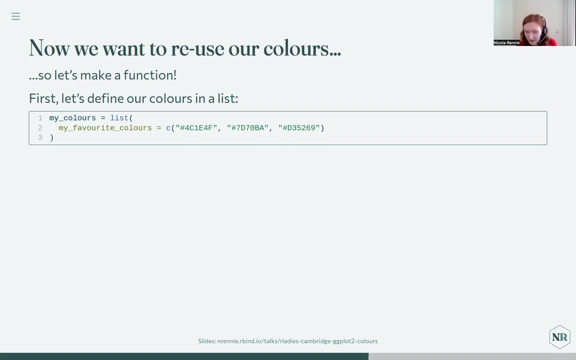 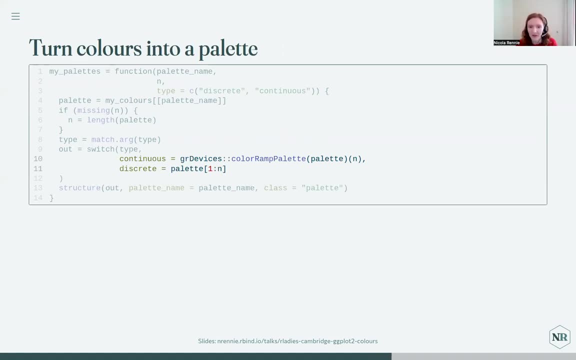 called it my favorite colors, Then we need to somehow turn this list into a palette object, in the same way that when you use scale functions with the sort of default colors in ggplot2, you'd never need to tell ggplot2 how to use scale functions. 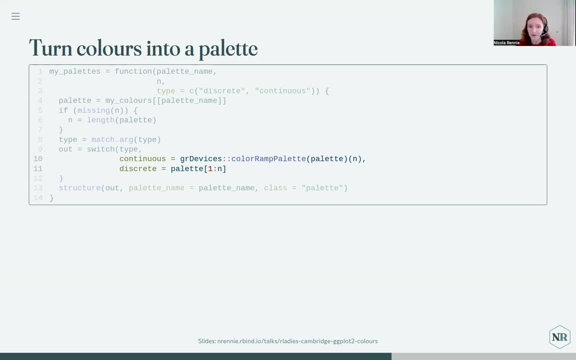 It sort of automatically calculates it for you. We didn't need to specify that we needed three colors to go with the three species of lemur, like we did with scale manual. the sort of default ggplot2 functions know how to do that. I won't go. 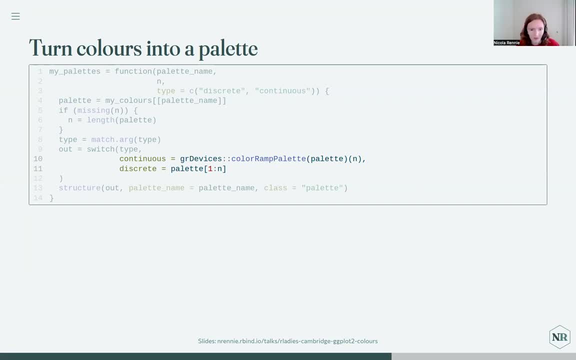 through all of the codes for this sort of my palettes function here. it is available online if you want it. but the important thing to point out here is I have two different outputs. I have a discrete and I have a continuous palette. so this will either give me a sort of 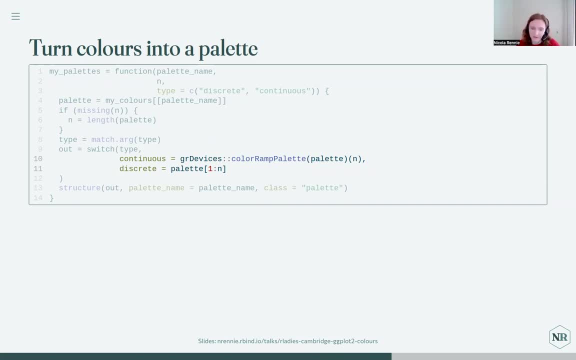 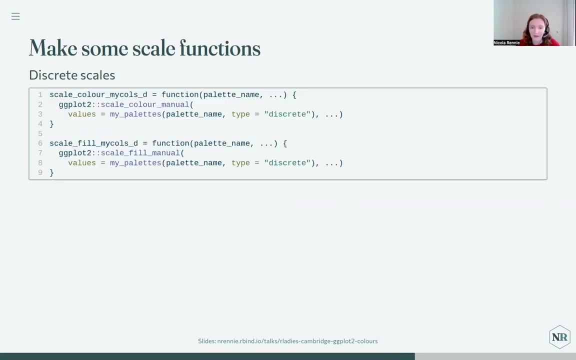 color gradient bar or a discrete legend and we can check if it works. If we use this palettes function, select the name of the my favorite colors palette. it gives me the vector of colors back and now we can make our scale functions so for discrete colors, these are just a wrapper around the scale manual functions. 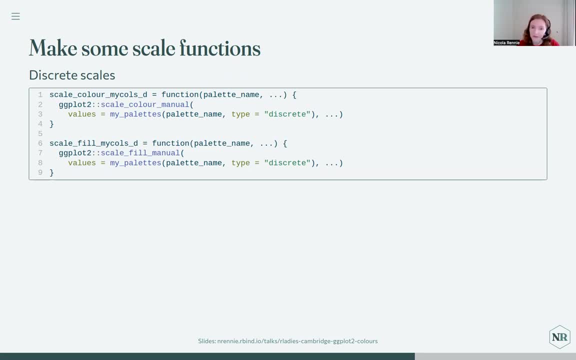 and I just put in the palettes function we just created, to the values of colors. and here one important thing is sort of adding in these ellipses here, and that means that you can use any arguments that you apply to the scale manual functions in your new custom scale functions as well. You inherit those. 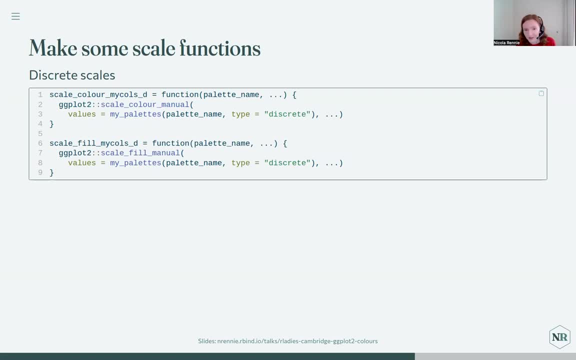 arguments. so, for example, if you want to change the legend name or setting the limits of the scale, you can still do that, but you don't have to change the values. so you can do that automatically with this new scale color. my calls function here. Continuous scales have a very similar idea. so here, instead of 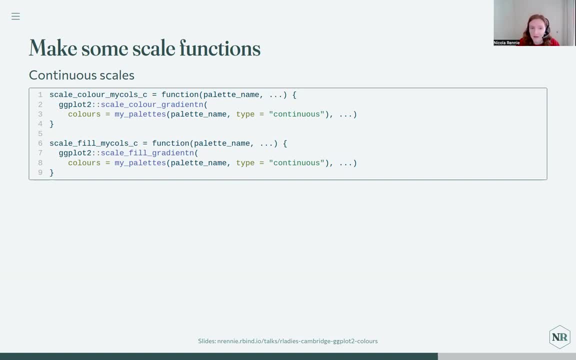 wrapping around scale manual. we wrap around scale gradient n. so this function sort of interpolates the n colors you pass in into a continuous color bar and we have the same thing with the ellipses here as well. so if you want to match sort of limits or break points in in your 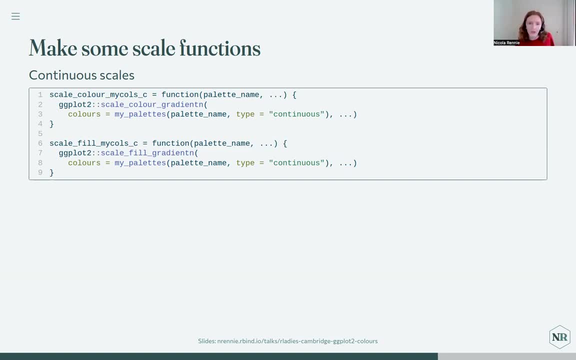 scale. you can do that as well If you want to match ggplot2. you can also make sure your functions work with either the American or British spelling of the word color. you can just sort of reassign one function to the other. you don't need to. 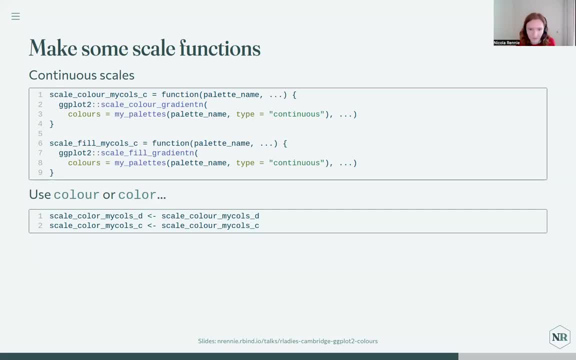 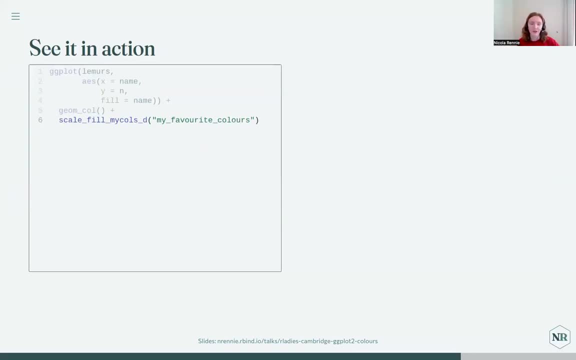 copy and paste two versions of it. So let's see it in action. just back to more lemurs. okay, so this time we're using our custom scale function and we get the same plot as when we used scale manual, but here our work has less copying and pasting. it's easier to use. I don't need. 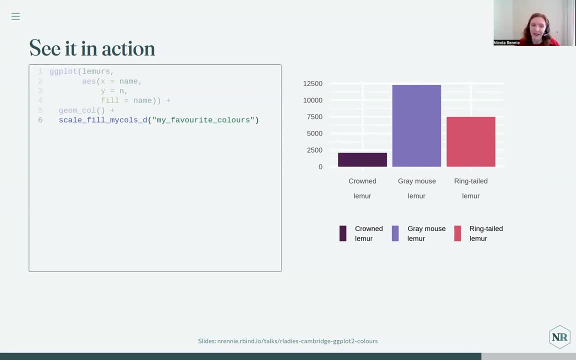 to specify that I needed. I don't need to manually count out the three colors, I can just use my function, and ggplot2 does it automatically. and if we were to color by n- the number of lemurs, so a continuous variable- instead we could use our custom continuous scale. so here I've also changed the limits and the. 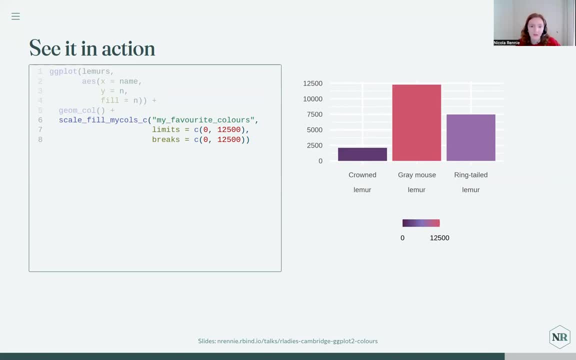 break points in the color bar scale to show you how those inherited arguments work, and we get our continuous gradient here instead. So let's say you've done all of that, what? what do you do next? Okay, one thing you might want to do is define a print method. okay, so I've 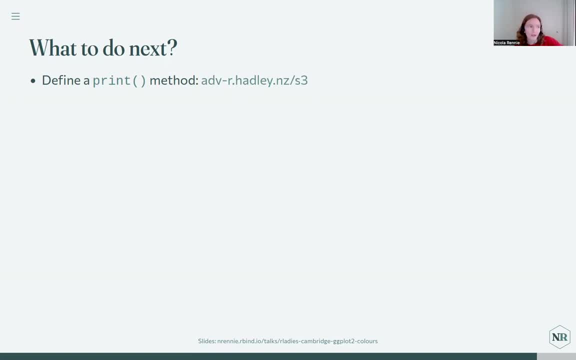 linked to the advanced R book here that talks about S3 methods. so when you're deciding which palette to use, it's usually easier if you can actually see the colors themselves, rather than just getting this vector of hex codes, because you don't really know what they look like if you just see them and then you 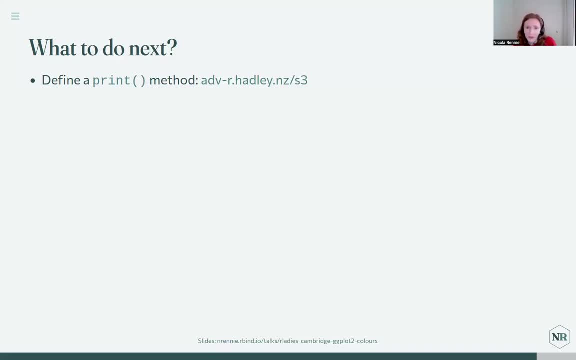 see the hex codes themselves. so what you could do is you could create a print method so that when you run your sort of my palettes function it prints the colors to the plot pane automatically and you can sort of visually compare them and decide which ones you want to use. The other thing that you might want: 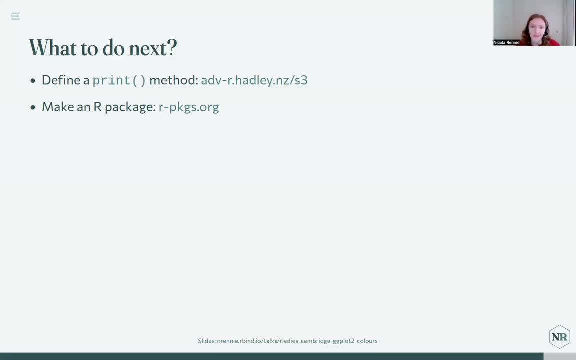 to do once you've made a print method is: well, we've just created a bunch of colors that we probably want to reuse either in our own work or we want to share them with other people, for them to use the same functions and palettes as I am, and that's normally an indication that you want to bundle them up into an.